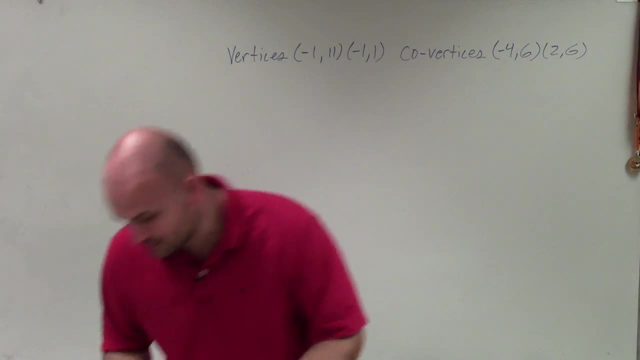 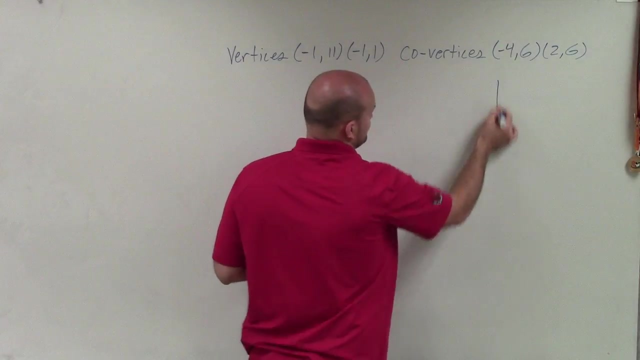 major axis and one with a vertical major axis. So we need to be able to determine which formula we're going to be using. So to do that, what I like to do is plot the points that we're given. Now remember, when we plot the points, that the center, the foci and the vertices 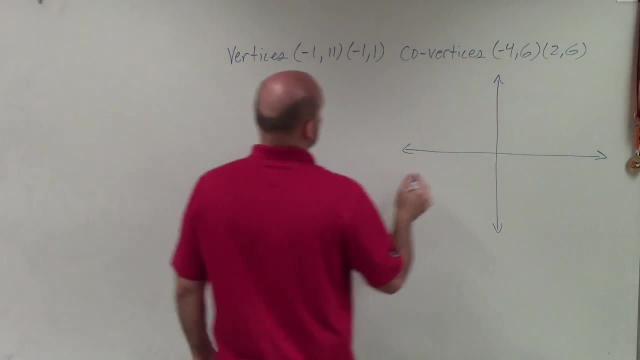 all lie on the major axis. So when plotting my points, I have negative 1, 11, negative 1, 1, 2, 3,, 4,, 5, 6,, 7,, 8,, 9,, 10,, 11.. And I have negative 1, 1.. So those are my two vertices. 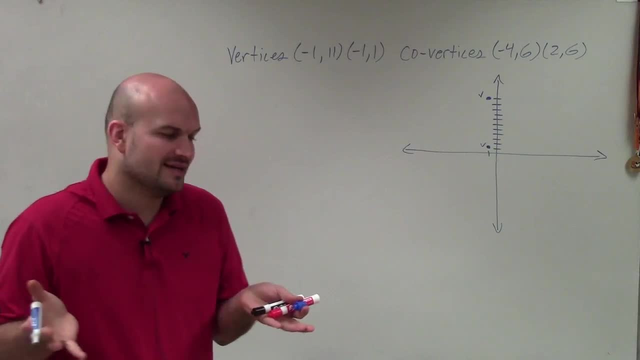 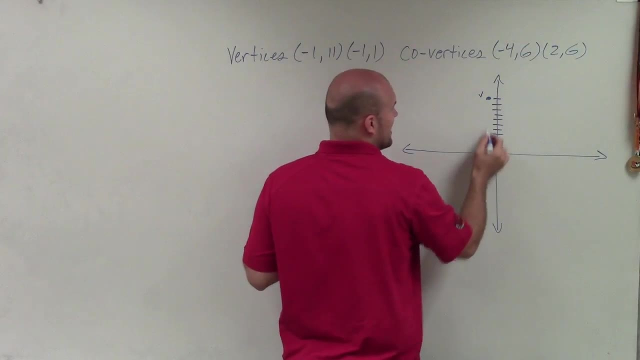 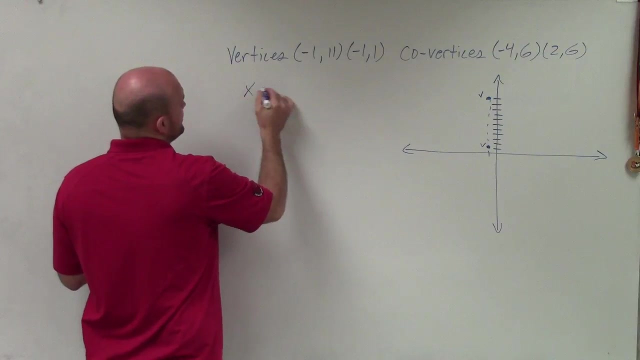 Now, without even graphing, without even finding my co-vertices, I can see that, since my vertices have to lie on the major axis, I can see that my major axis is going to be vertical, right? So therefore, I'm automatically going to use the formula. 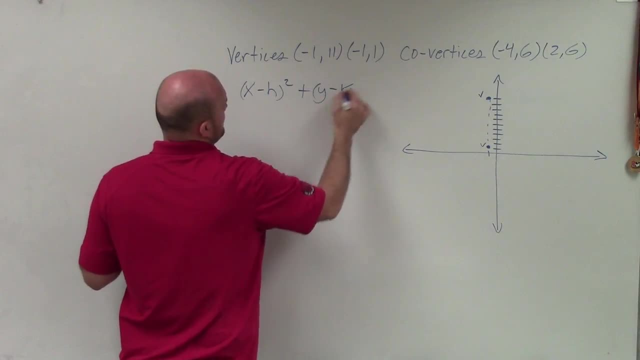 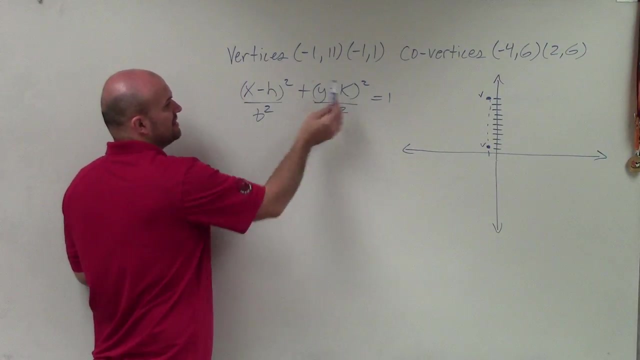 x minus h squared plus y minus k squared, equals 1.. And then remember, when it's vertical, the a, the distance from my center to my vertices, is going to be the y, and my b squared is under my x. So now my idea is going to be to figure out, find a, find b and find yk. 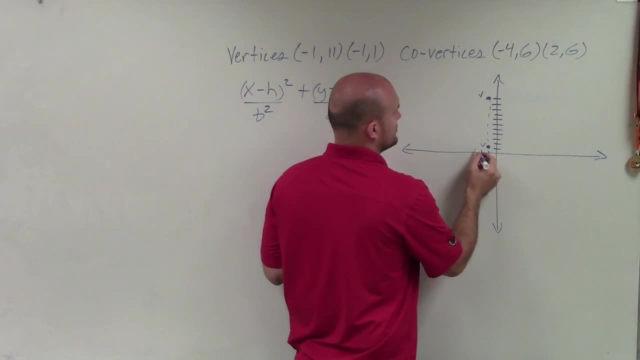 Let's plot the co-vertices though first. So that's at negative 4,, 1,, 2,, 3,, 4, up 6.. 1,, 2,, 3,, 4,, 5,, 6.. And at 2, 6, 1, 2, up 6.. 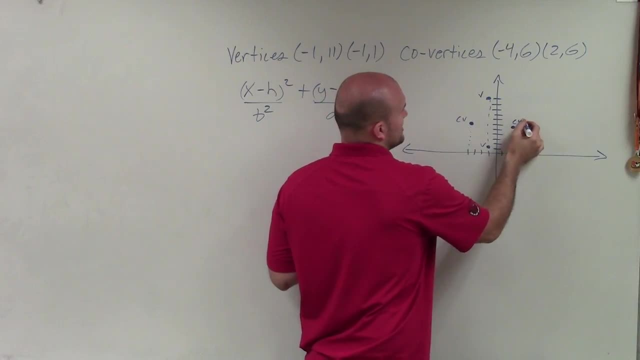 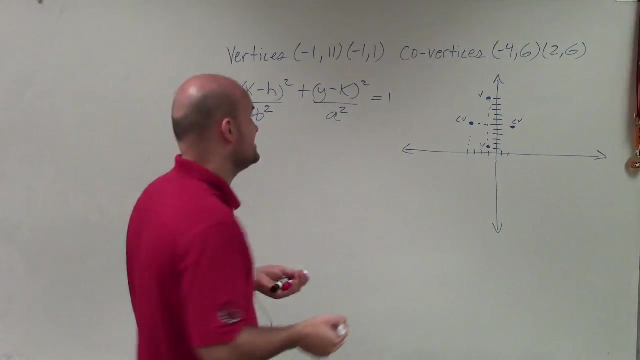 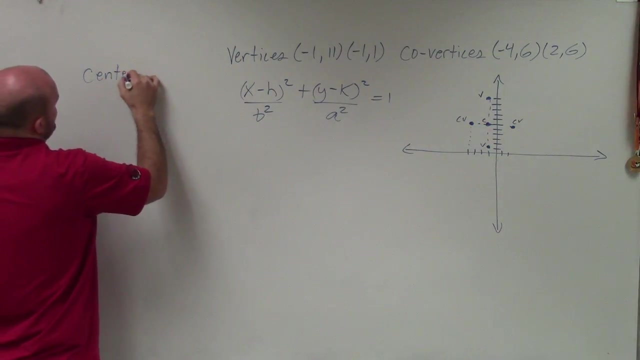 Okay, now what's important. so this is going to be, these are my co-vertices and these are going to be my minor axis as well. Now notice that the intersection of the major and the minor axis is going to be the center, which will be right here, So I can see the center. let's just kind of write in our information: 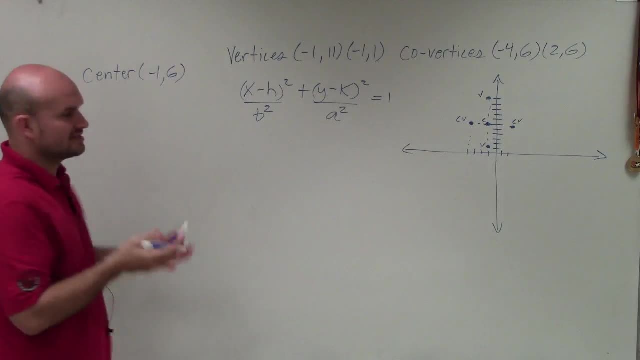 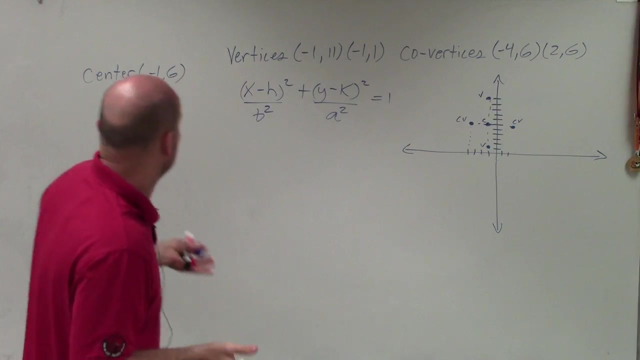 the center is going to be at negative 1,, 6, because it's going to be in between the, or it's going to be at the intersection of my co-vertices and vertices Now. so remember, the center is always in the form. 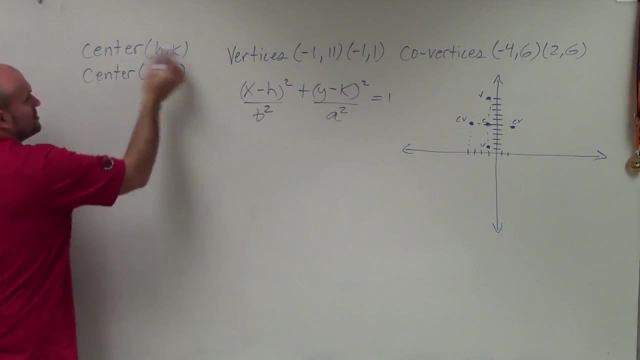 of h- k. So therefore I can determine that my h is negative 1, and my k is 6.. Before I enter those in, let's go ahead and figure out what my a and b are going to be Now. remember a is equal to the distance. 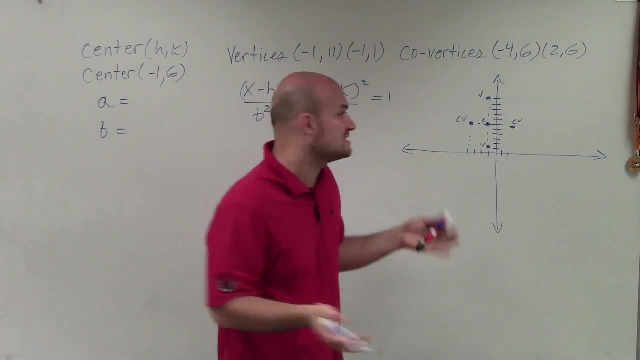 which is going to be at negative 1,, 6, because it's going to be in between the, or it's going to be at the intersection of my co-vertices and vertices, from the center to either one of the vertices and it's an absolute distance. So all I need to do is go from my center and go up to my. 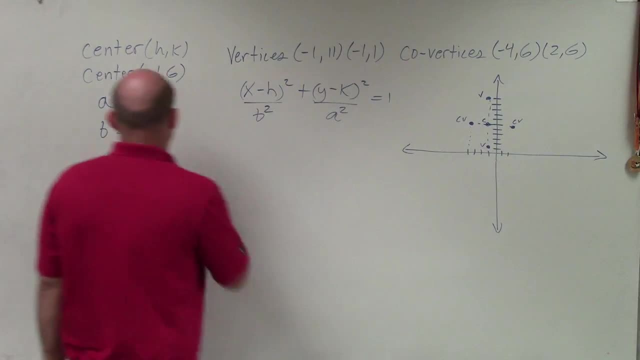 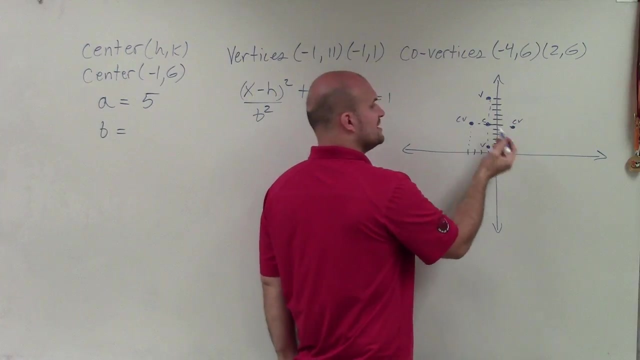 vertice which is 1,, 2,, 3,, 4,, 5.. So therefore, I can say a is 5, and I can just double check that, going in the opposite direction: 1, 2,, 3,, 4,, 5,. good, And then my co-vertices is going to be or, I'm sorry, b is going to be. 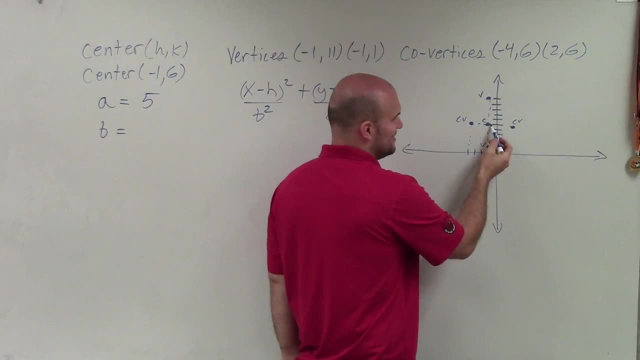 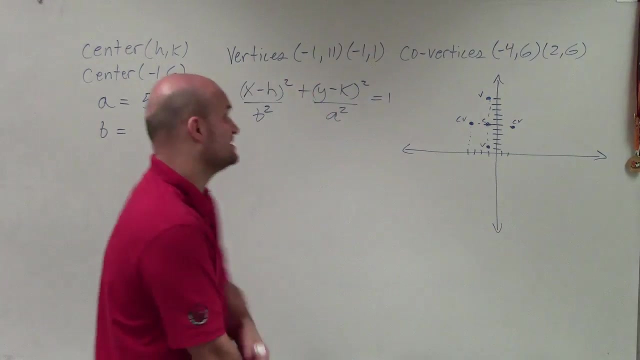 distance from my co-vertice to my center- and I know it kind of looks a little awkward here. Let's make sure 1, 2, 3,, 1, 2, 3.. So I just kind of have a bad scale, but you can see that the distance from the center to the co-vertice 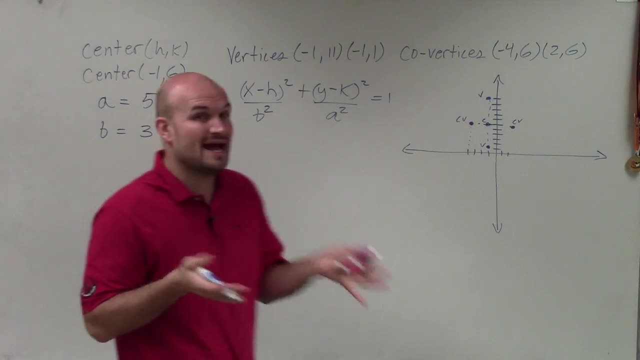 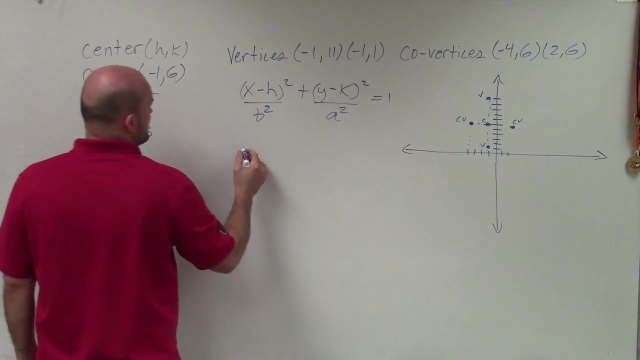 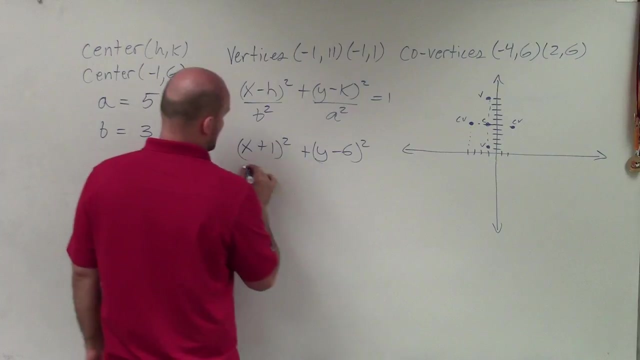 is going to be 3.. So now I know what a, I know what b is and I know what h, k is. so now I just need to plug them into my formula. Now remember, the formula is opposite of h, opposite of k, So it's going to be x plus 1 squared plus y minus 6 squared.